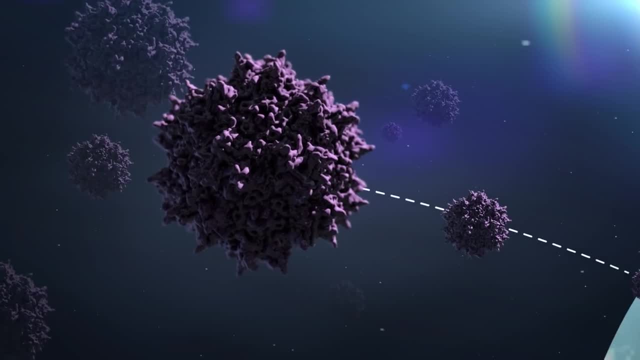 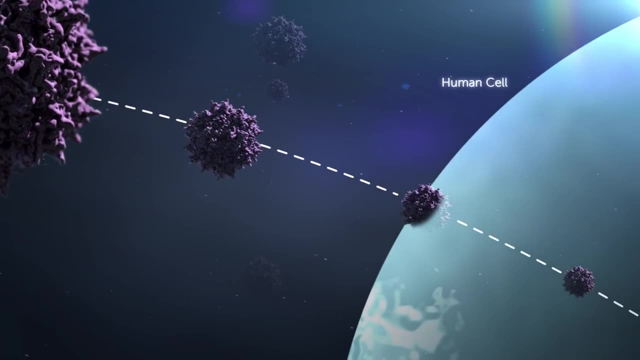 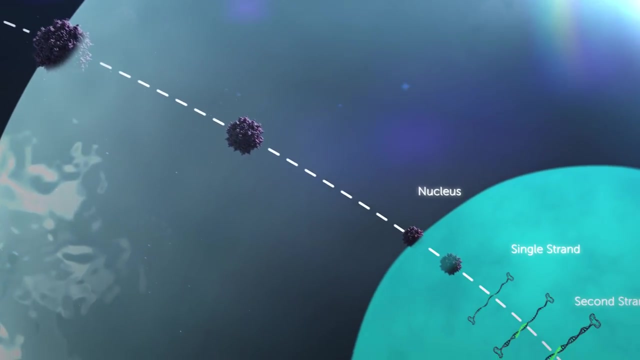 AAV vectors are delivered to cells in the retina by routine ophthalmic delivery methods such as intravitreal or subretinal injection. Once administered, AAV vectors enter the patient's cells and deliver a copy of the functional gene directly into the nucleus. 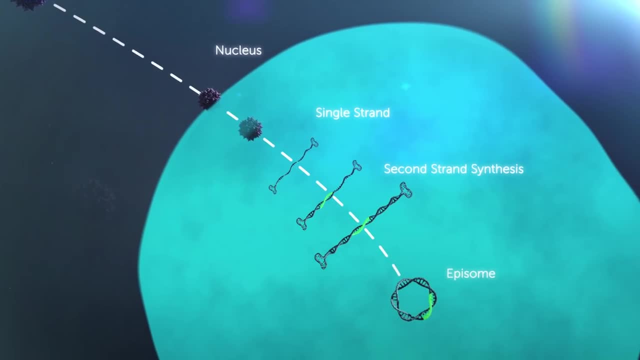 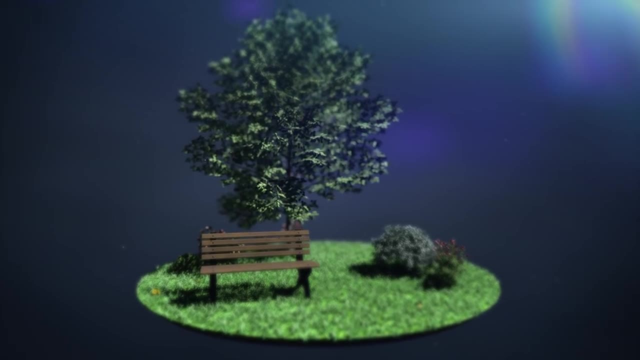 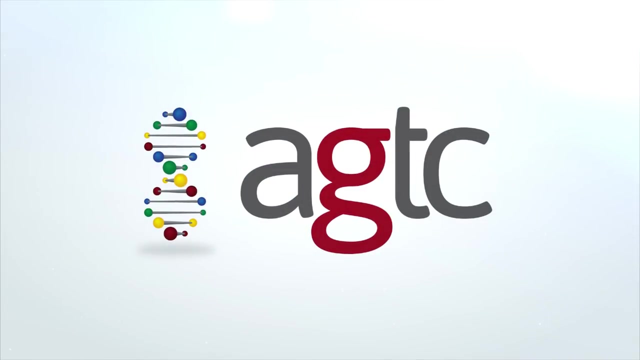 Once inside the nucleus, the functional gene can support the production of the normal protein and correct the underlying cause of the disease. Genetic defects in the eye can cause vision loss or blindness, and gene therapy can provide a long-lasting therapeutic benefit. AGTC is using its technology. 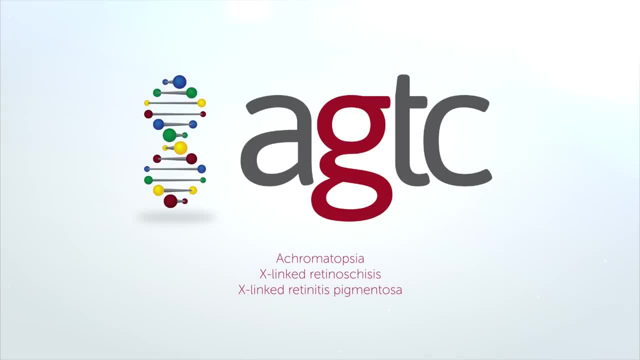 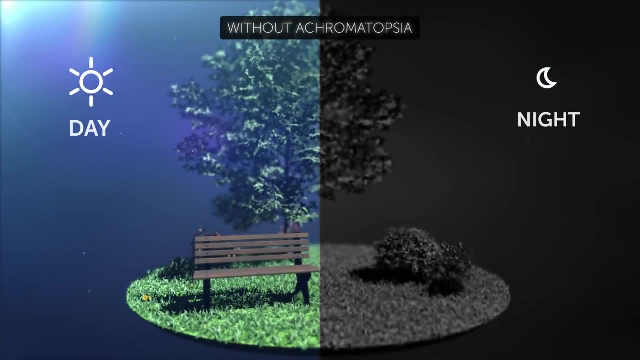 to develop gene therapies for rare inherited retinal diseases that currently have no treatments. One of these diseases is achromatopsia, an inherited retinal disease which is present from birth. Achromatopsia results in markedly reduced visual acuity. 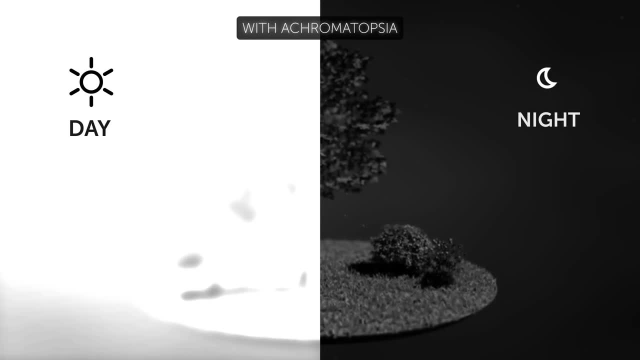 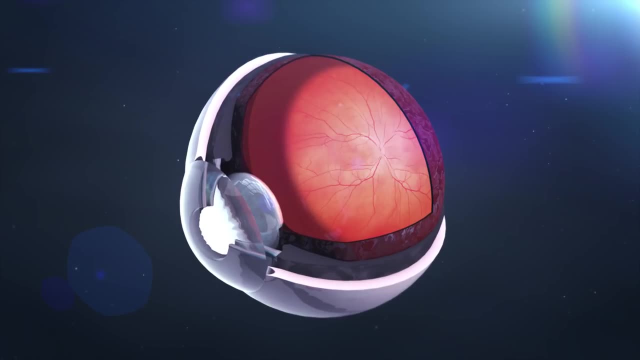 extreme light sensitivity causing day blindness and complete loss of color discrimination. The retina is a layer of cells at the back of the eye. In a healthy eye without achromatopsia, special cells in the eye called cone photoreceptors. 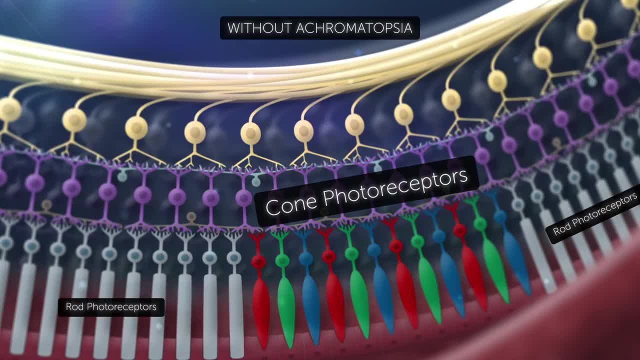 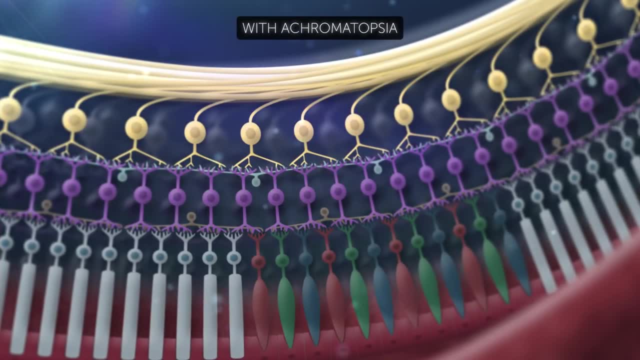 convert light into an electrical signal which is transmitted across the layers of the retina and then to the brain for visual processing. In an eye with achromatopsia, cone photoreceptors in the retina are unable to convert light into an electrical signal. 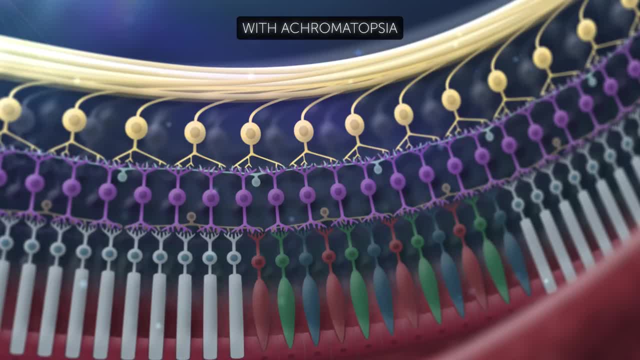 The most common causes are mutations in one of two genes called CNGB3 and CNGA3.. In gene therapy, an AAV vector containing a normal CNGB3 or CNGA3 gene is designed to provide the instructions for normal CNGB3 or CNGA3 protein. 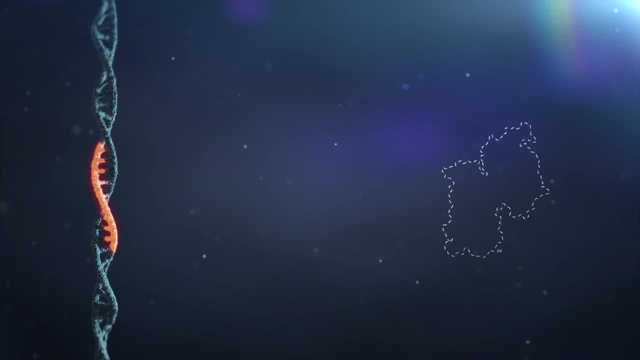 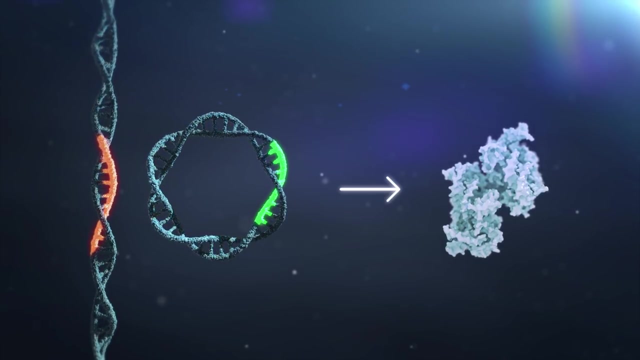 and restore cone photoreceptor function. By introducing a functional copy of a gene into a patient's cells, gene therapy is able to correct the underlying genetic defect that is causing disease. The functional gene delivered by an AAV vector is thought to remain stable. 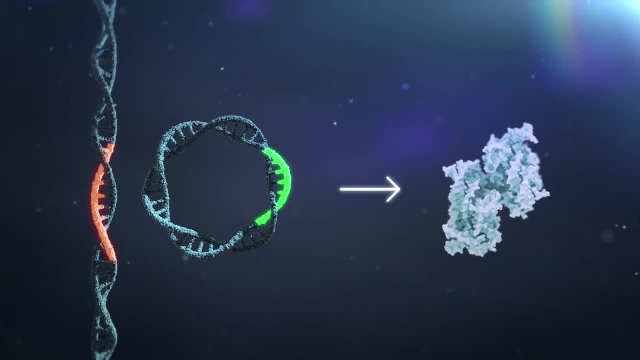 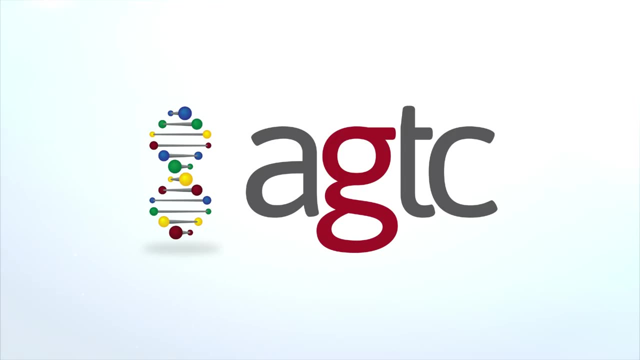 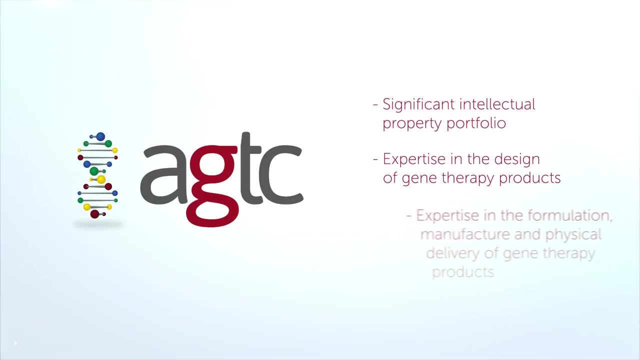 for many years, which suggests that gene therapy has the potential for long-lasting clinical benefits after a one-time administration of the vector. AGTC has a significant intellectual property portfolio, expertise in the design of gene therapy products and expertise in the formulation manufacture.